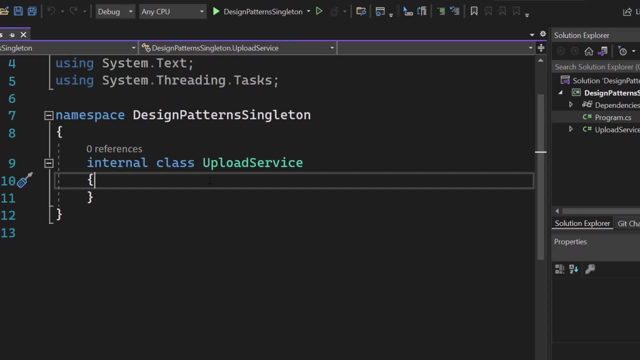 convention. So let's just assume that we want to create any kind of functionality and I decided to stick around with an UploadService, So something that uploads something to the internet or something like that, and we want to have that class as a singleton implemented. 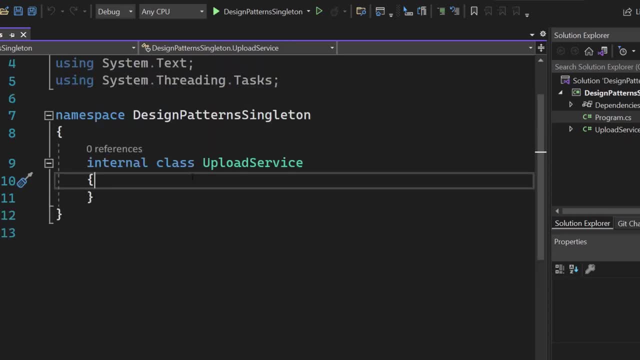 Now let's talk about the word singleton first. So singleton means that you can only have a single instance of that class to be created. right, Singleton single makes sense. So if we have one instance of the UploadService, then there can not be another one. That's the singleton design. 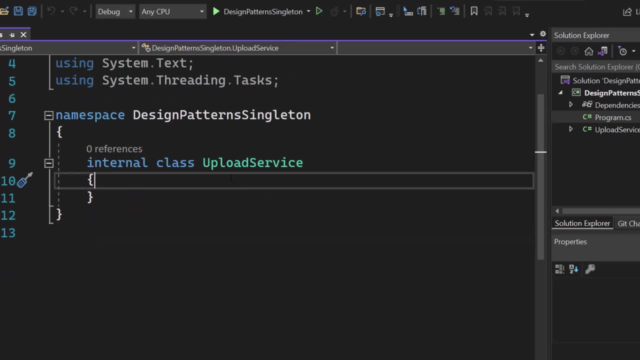 pattern. So there is one important information that you should know about the singleton design pattern, and it is that we have to make it thread safe, and you will learn what that means and how to do it during the video. Alrighty, so let's get started. Let's turn this internal class here. 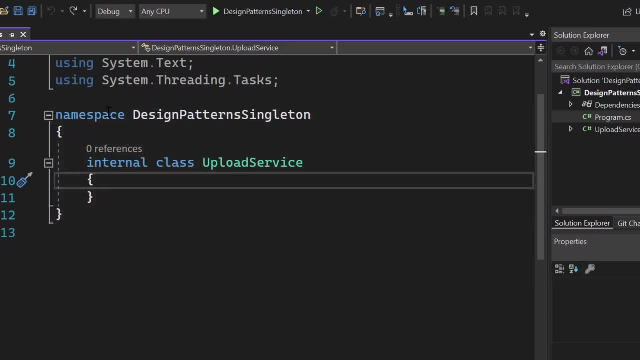 that I just have created into a singleton. Okay, so here we got our internal class. The first thing that I want to do is I want to remove the internal. We will just replace that with another keyword in a second. Let's get started by creating a constructor. So simply. 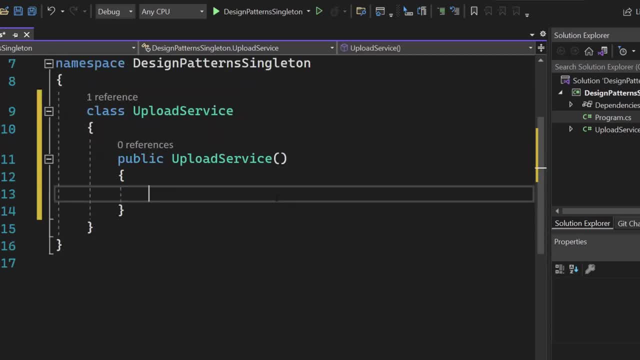 write down ctor and hit TabTab. Now best practice is not to add any kind of parameters, because that's against the pattern. If you would need any parameters, then a singleton is not really what you're looking for, because a parameter for sure can be variable, but we only want to have 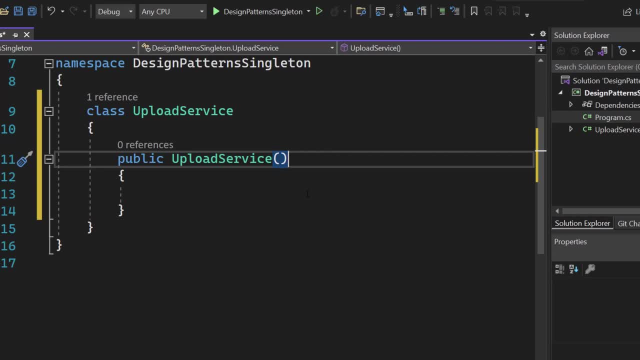 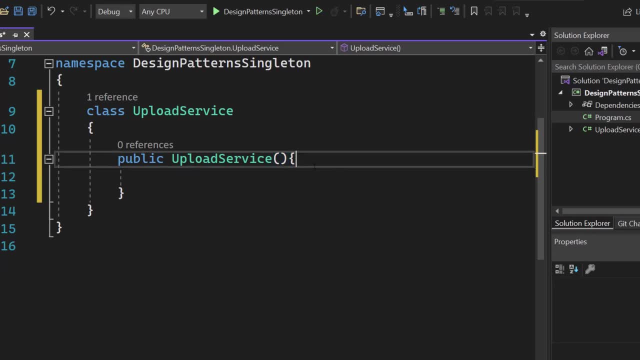 want to keep that constructor here empty. So we want to keep that constructor here empty. Now, let me shorten that up. Let me shorten that up, Let me bring that into a single line of code here, so that we don't want to add anything. And, very important, we want to switch that not from being 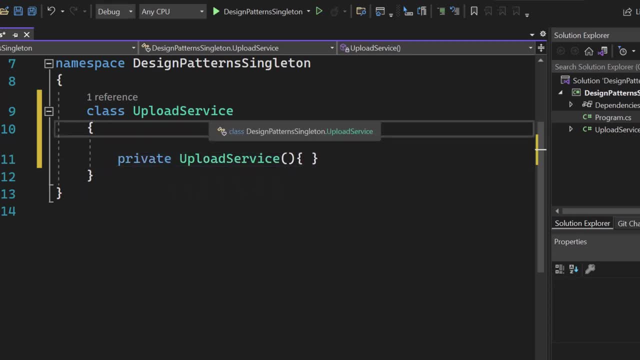 public but private instead, because only the class itself should be able to create an instance. So we should not be able to create instances of that upload service from outside of this class, because well, that's against the singleton pattern. If any other class from outside here could create an instance, then we could not. 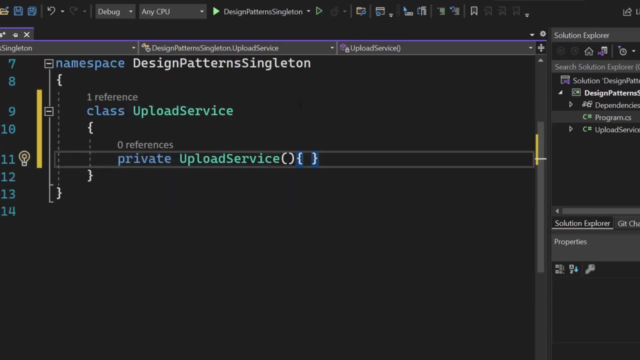 be sure that only a single instance of that service exists. Now, next up, we want to add a reference to the actual instance. This is why we add a private static. very important. make it static. Let's call it upload service, right, Because? 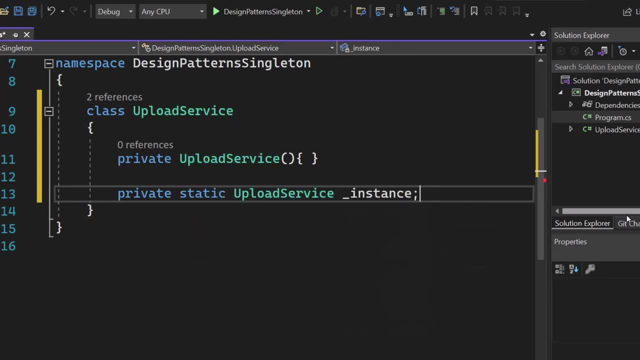 the instances of this type and let's call it instance. Now we make it private because in a second we will create a static method which gives us the information about the instance. So we can make a private here And we make it static so that we don't need any instance. 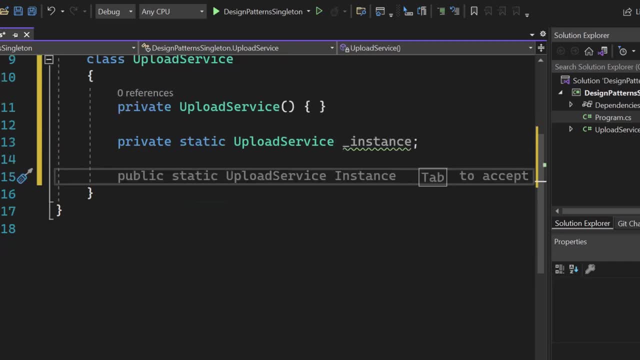 to have a singleton instance. So now let's write down a method which gives us the information about the instance. You want to call that method to get the instance. Actually, we want to make it public, We want to make it static And for sure it returns the upload service. 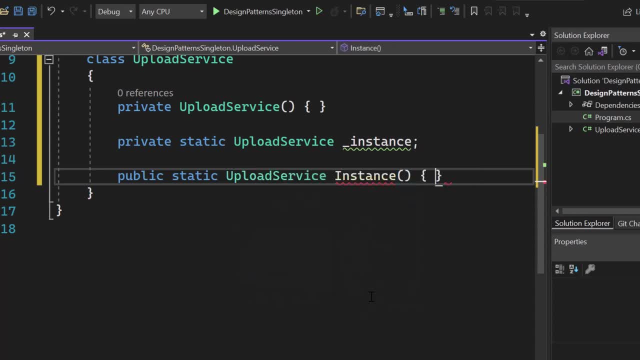 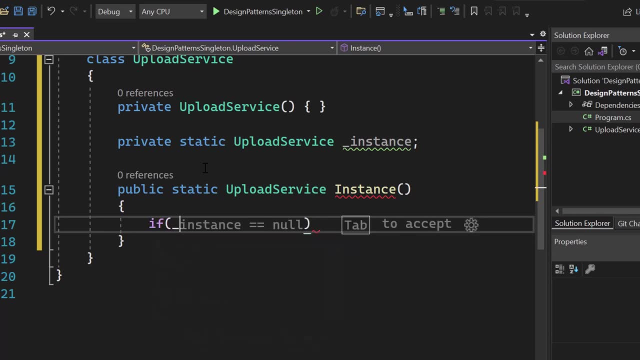 And then let's call it instance: Awesome, Great. Now the basic code behind this- you can see that already suggested here- is like: if the instance that I have here in line 13, if that instance is null, so if it's equals to null, so if we don't have 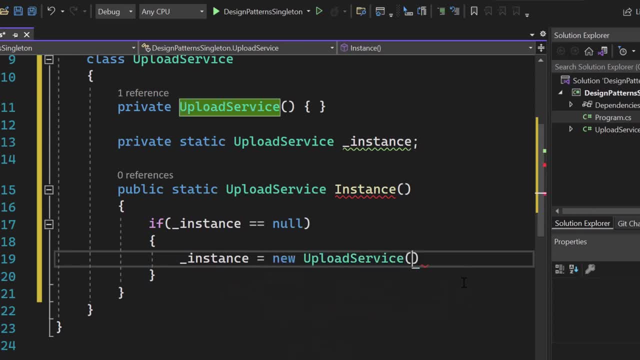 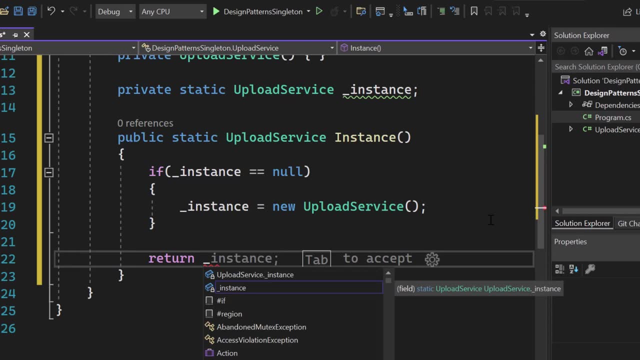 an instance, we want to create one. So new upload service, right? So if we don't have an instance, create an instance. And now, finally, we want to return something from that method And for sure, we want to return the instance. Awesome. So basically, this would be a very simplified 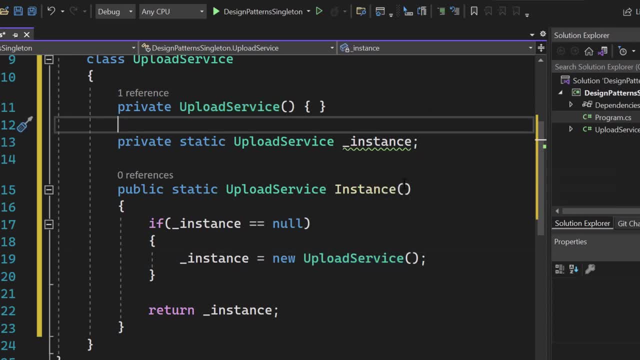 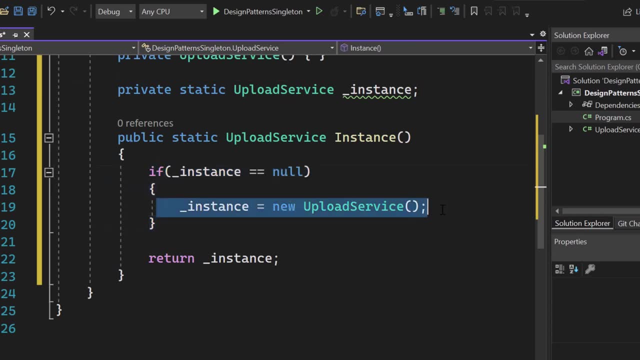 version of a singleton, It would be already working. There's this one problem, However. as you can see, from a logical side of view, that will work. We don't have an instance, we create one. But if we have an instance so that one will not become true, the if statement will become false, right. 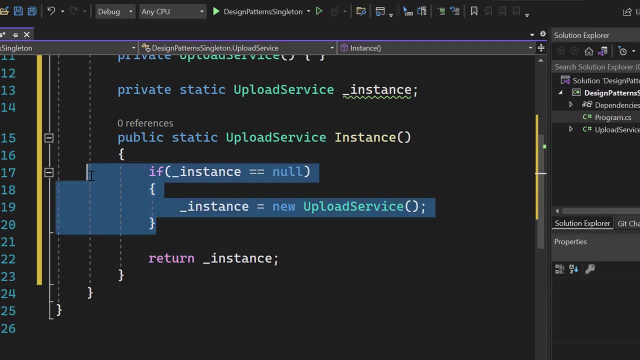 And we will directly return the existing instance. So if we don't have an instance, we create a new one. If we have an instance, we simply return the existing one. Awesome. So the next part of this video is really very, very important. But before we get to that, make sure to subscribe. 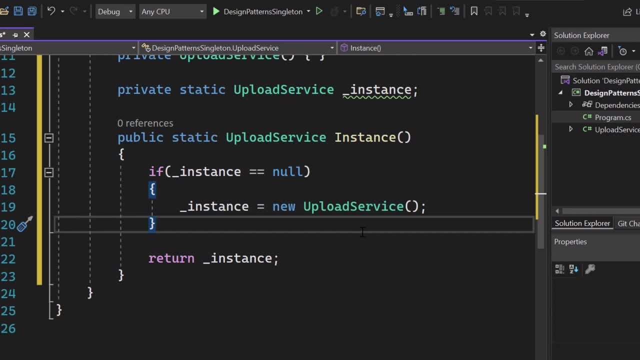 to our channel so that you no longer miss any upcoming dotnet related videos And if this video helps you out and you like it, make sure to give it a thumbs up to support our channel And so that we know what content you really want to see. Oh and, by the way, we got an online course. 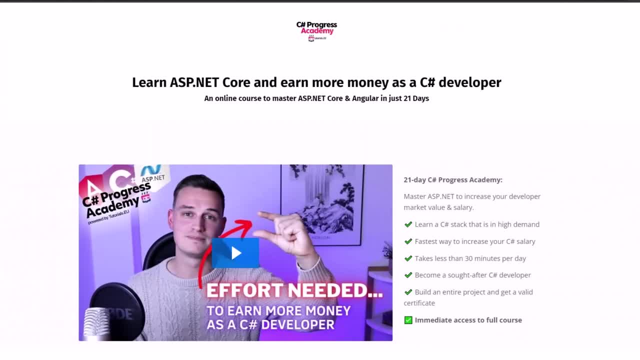 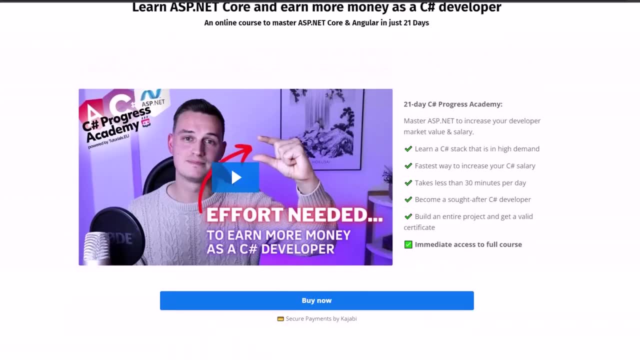 a very unique online course. we call it the C sharp Progress Academy. Well, it teaches you ASPNET, Core, Angular software, design patterns and test driven development Basically in 21 days. you can go through it in your own speed And I'm absolutely. 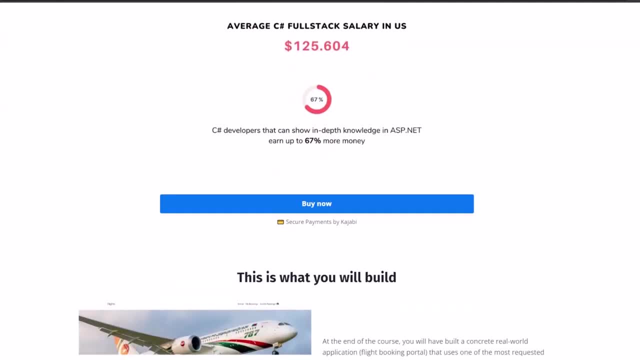 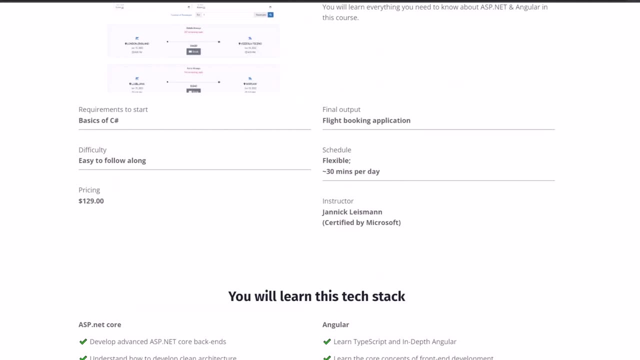 sure about that. this is the fastest way to become a better C sharp developer. So if you really want become a dotnet hero, check out our c-sharp progress academy. you can find the link in the description below or in the info card popping up right now. great, so now let's get to the second. 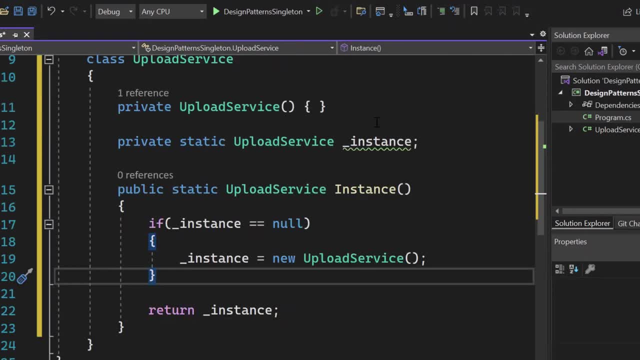 part of this video. basically, even though this pattern here is working right now, it's pretty simplified because in real world we need to create a singleton pattern which is thread safe. so as long as you only have a single thread in your application, this pattern here is fine. but if you 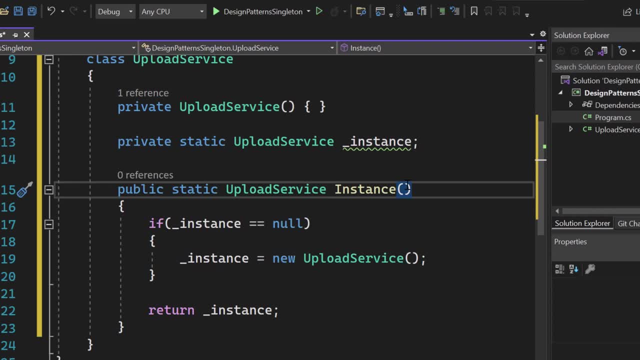 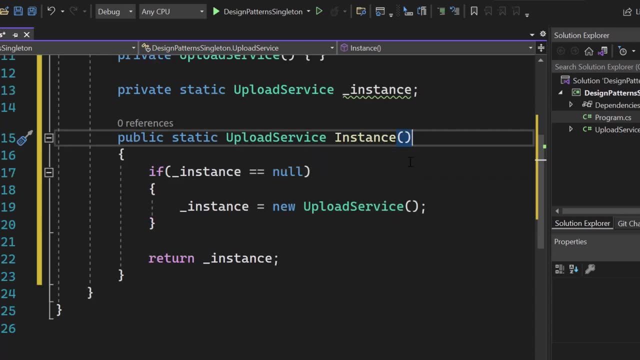 have a multi-threaded application, we need to make sure that we add a log here so that another thread is not creating a new instance again when we start the program. so basically, so that you get the ideas, like if we have multiple threads and we start the application and those threads are starting. 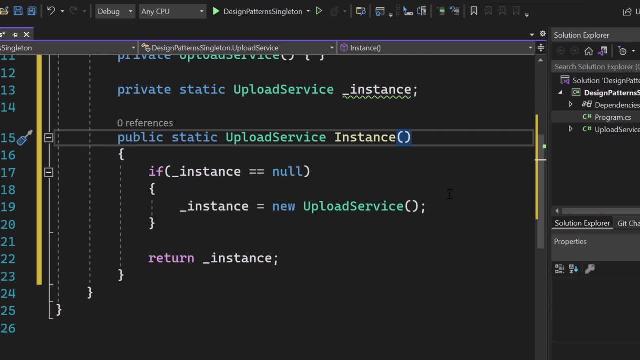 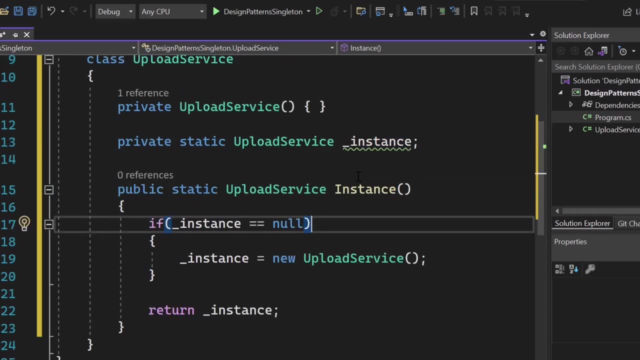 we need to make sure that only one thread is creating the instance and not another thread is also creating one because it sees like: okay, the instance is not and this is why we use the keyword log. so we create a log object and then one thread will reach this position, the lock- and all other threads will wait until it's finished. but we 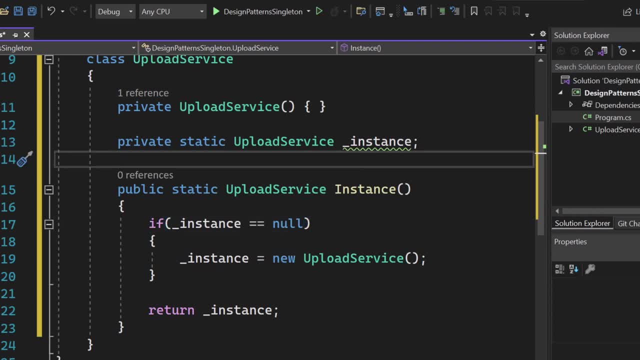 will see that in action. now it sounds more complicated than it is and it's really a nice practice and if you are a well seizure beginner or kind of intermediate, i'm pretty sure that you have never used the lock before now. let's see that in action. let's create a private static. 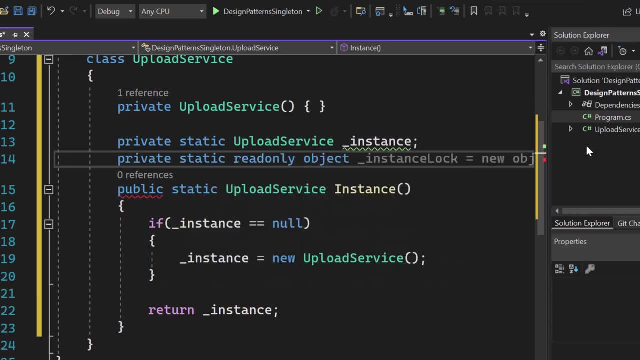 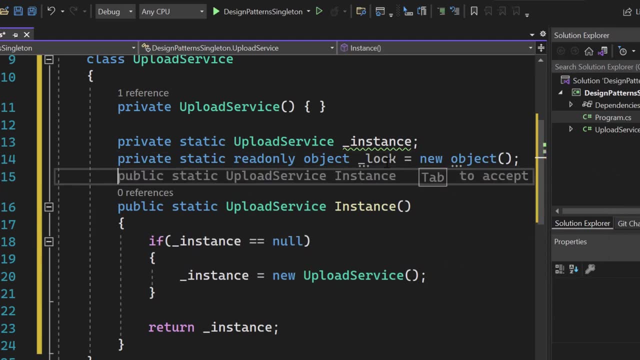 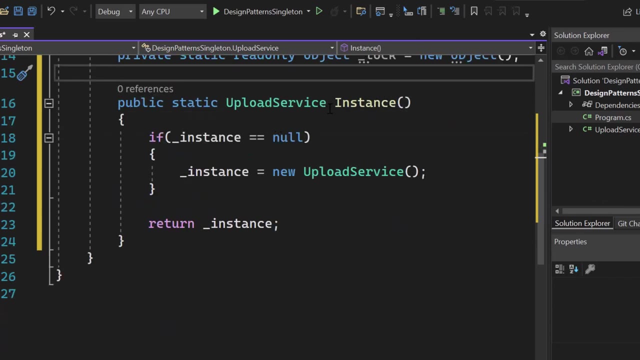 and read only object, and this one we call it lock and it's basically a new object. this is all what we have to do, right here. so just a simple static, read only object. now the magic happens inside of our instance creation. so right here, right at the position where the instance is null, right just. 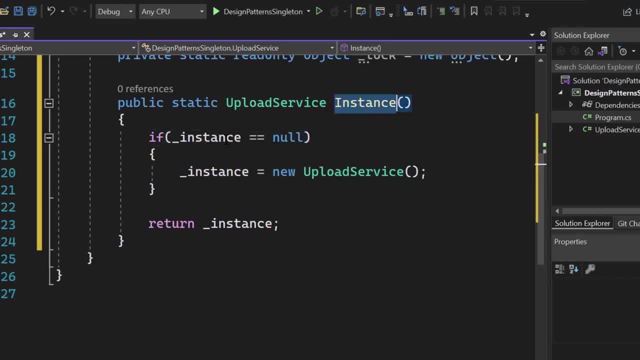 imagine that we have multiple threads which come into that instance method and they see: okay, the instance is null. so at the moment we start the program and the threads reach that position, the threads will see that the instance is null and multiple instances would get created and that's a. 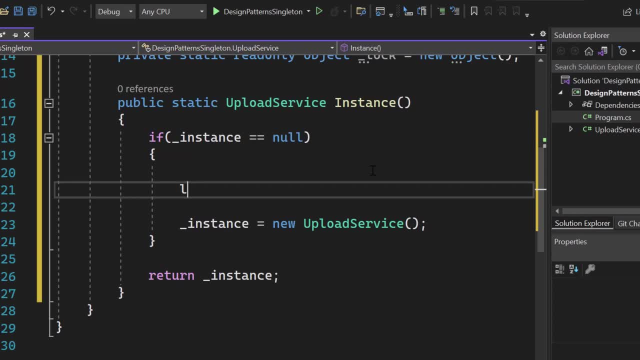 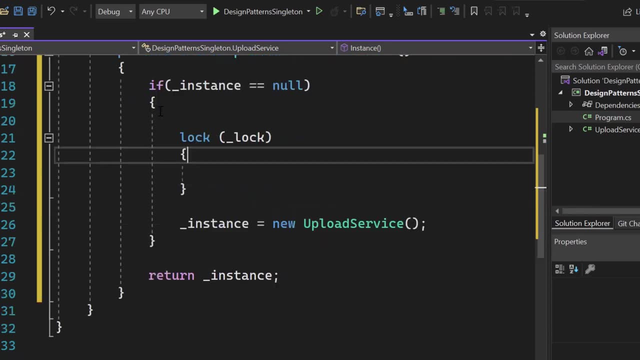 violation against the singleton pattern. so what we want to do is we want to use the lock keyword here and we want to lock and send in our lock object. now inside here we basically want to repeat the code that we have right here. so again inside the lock, i want to say: if instance is equals to null, then we want to create: 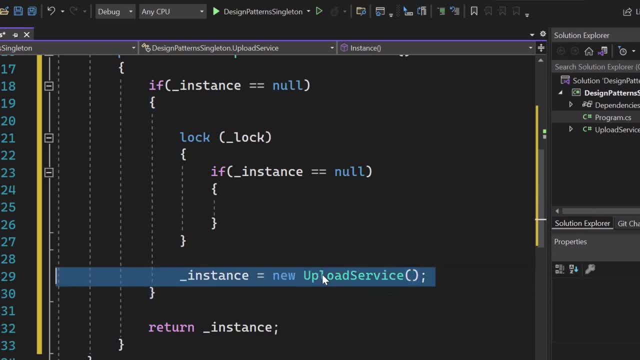 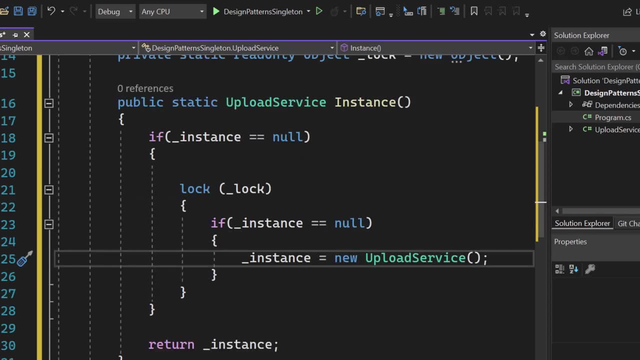 a new instance of that upload service. so take that line of code here, cut it out, paste it back in here and we're done. so let me explain that to you. so we start the program and both threads are done. so let me explain that to you. so we start the program and both threads are created and both threads are. 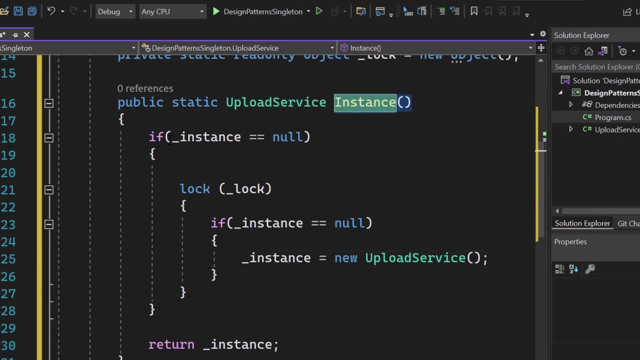 starting. they will come both into that instance method here they will both see that the instance is null because it doesn't didn't get created yet. so in the previous code both threads would now create an instance and that's wrong because we have a singleton pattern, so we only have a single. 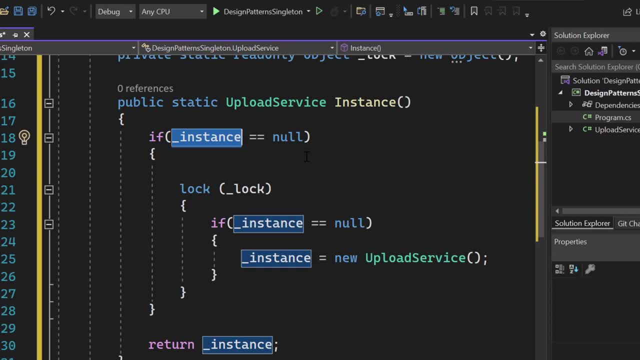 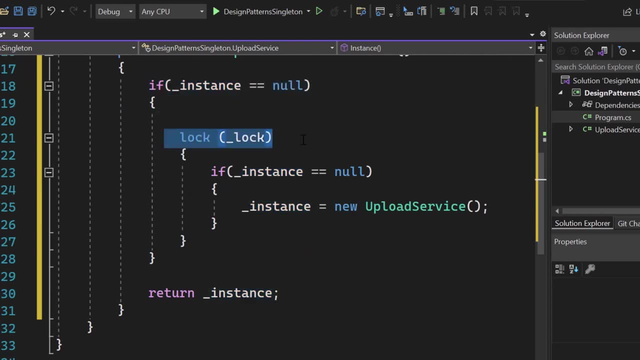 instance shared between all threads. the entire application only has one instance of it. so both threads are in line 18 right now. they will come to line 21 and the log keyword basically means that now a single thread will proceed through it while the other threads are waiting. so let's say thread one will work through this and thread two 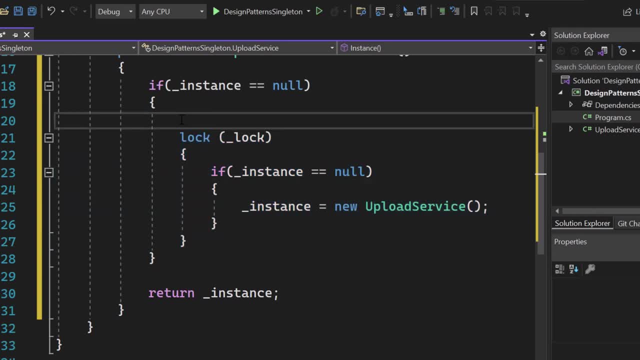 is waiting in line 20 until the first thread is done. so from the side of thread one, we will now go inside this code block. he will again see: instance is null. he will create an instance now. so now we have an instance in our application. okay, so we are done. let's switch over to the 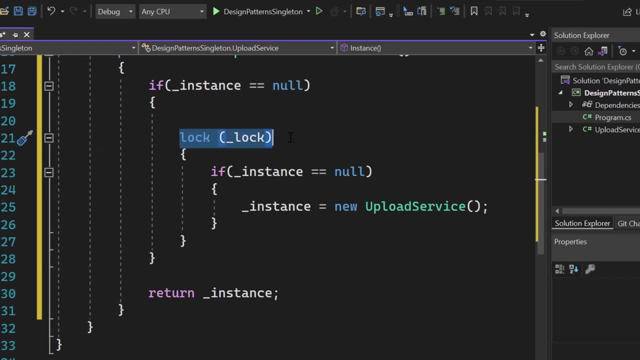 second one because he will wait at the log, or he's still waiting, but now thread one is done, so thread two will proceed from here. he will now take a look again. is the instance null? but no, the instance is not null anymore, because thread one created an instance and so the if statement will not become true, and instead he 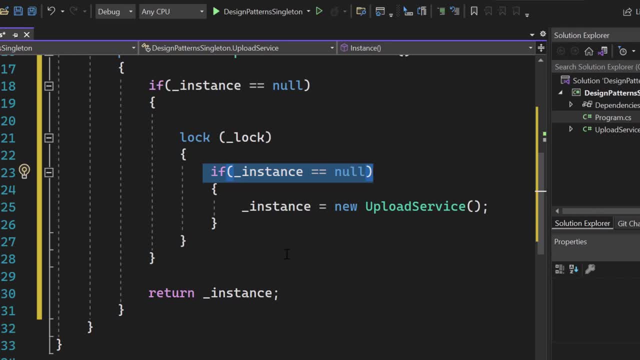 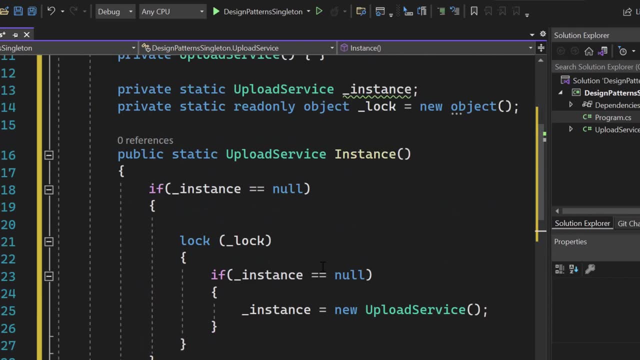 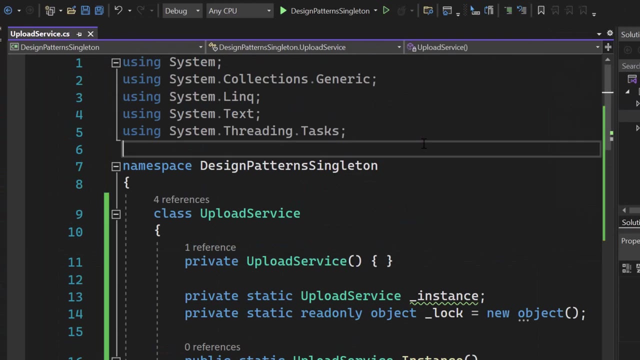 will know about the instance of the object which thread one has created, and he will simply end that if statement and return the existing instance. and in that way we have created or implemented a singleton software design pattern which is thread safe, alrighty. so now let's prove that this 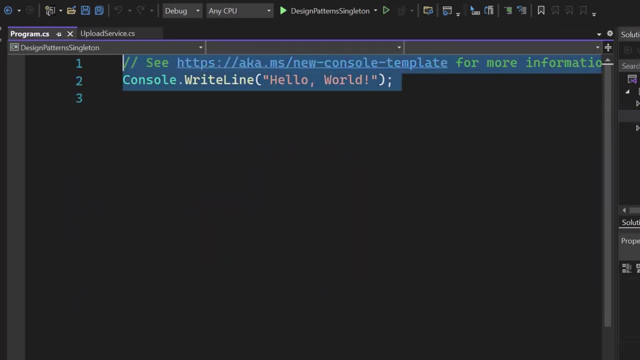 is actually working. let's switch over to our programcs and let's first of all start using our upload service here now. first things first, let's start using the system so that we are able to create threads, and that's what we want to do. we want to go ahead and we're going to create a thread here. so thread. 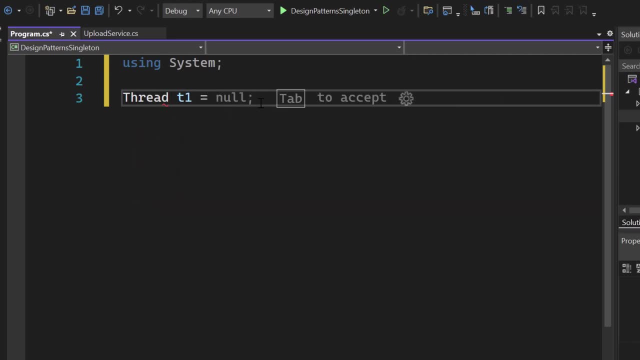 let's call it t1, just to keep it short- equals to a new thread, and inside that thread we want to go ahead and create a new. let's just do it that way, because i'm sure you can see the thread already separated out. so we want to get rid of that thread. 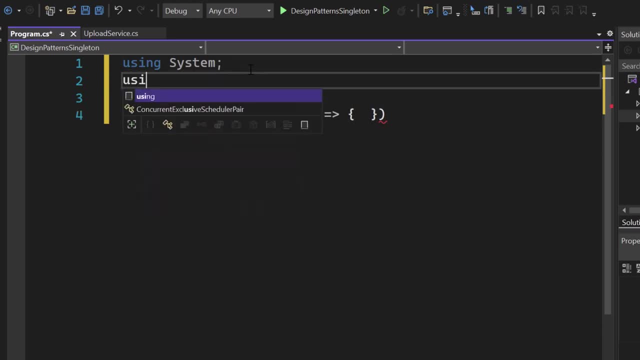 and we're going to do that right now, and we're going to give this a name function and we're going to call it a function- arrow function here- and we basically just want to run a single line of code. we want to call our upload service and for that we're gonna use the namespace design pattern. 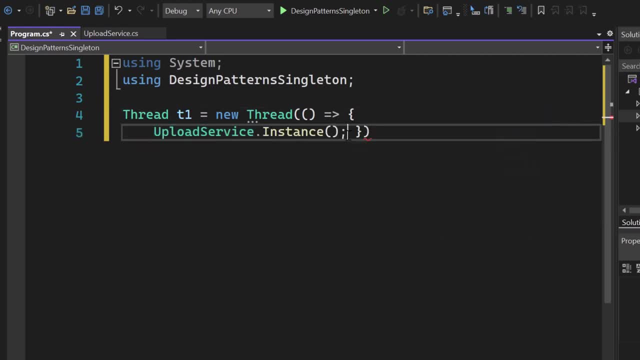 singleton. here. there we go, so that we get access to the service, and then we want to just call the upload service here, and we got a method inside of it which is called instance for sure. so let me just break that into another line of code. here we go, and let me add a breakpoint here. 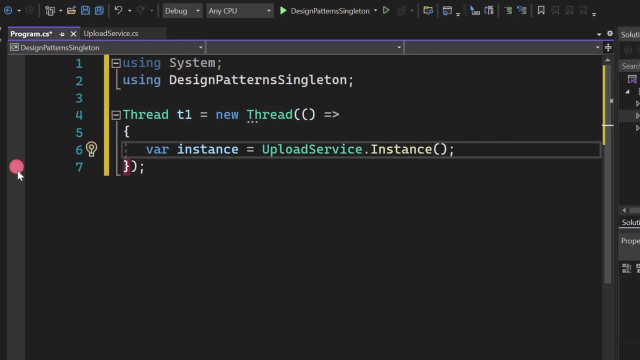 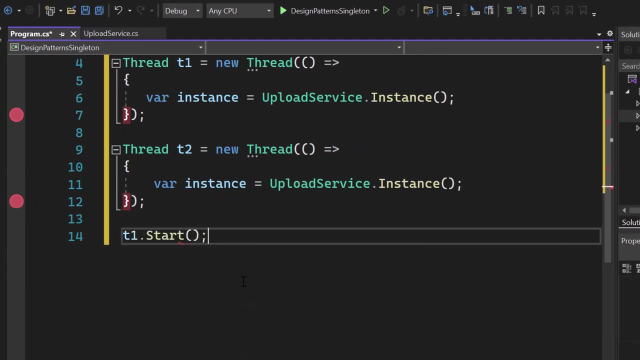 instance. there we go and I want to add a breakpoint here in line 7 and I want to copy that over and I want to go thread to the same stuff again. I want to add a breakpoint now. let's simply start both threads, so start both of them. very. 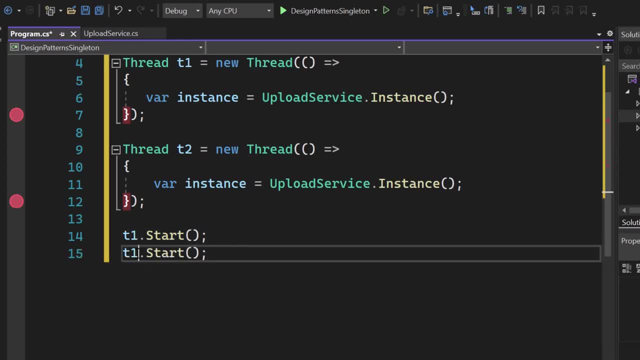 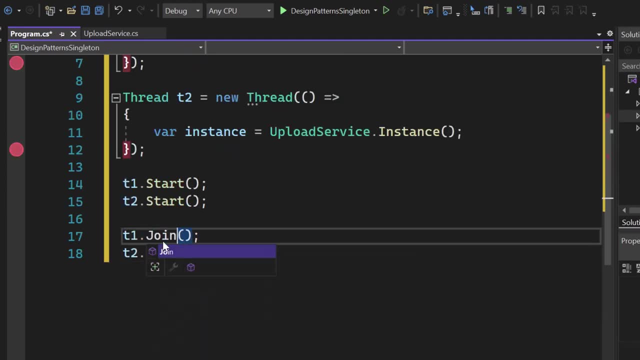 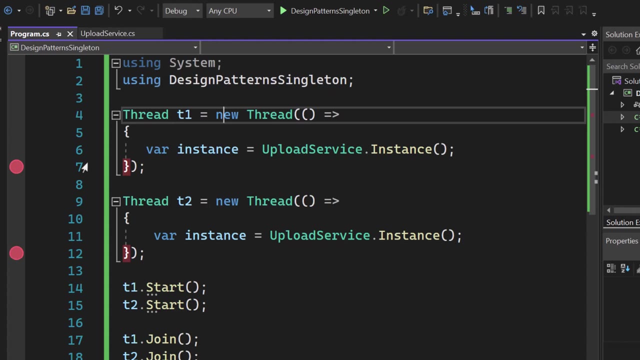 important that we do it in that order here, so that we're really able to test it in a valid way. and then we want to join. so t1, t2, starting them, joining them. there we go, and we want to have any kind of ID or something like that so that we 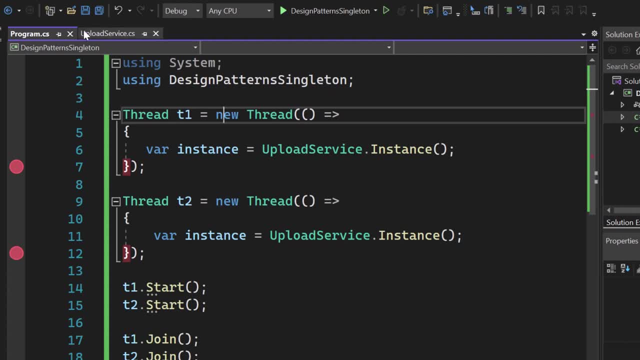 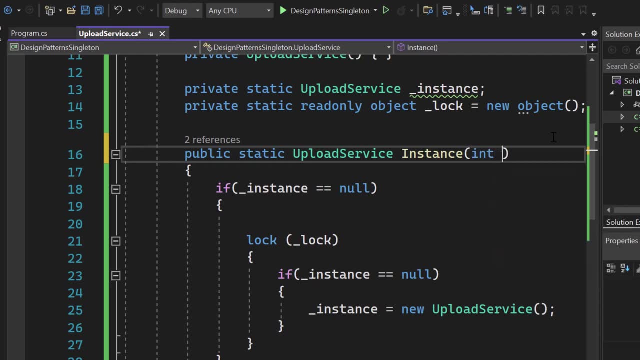 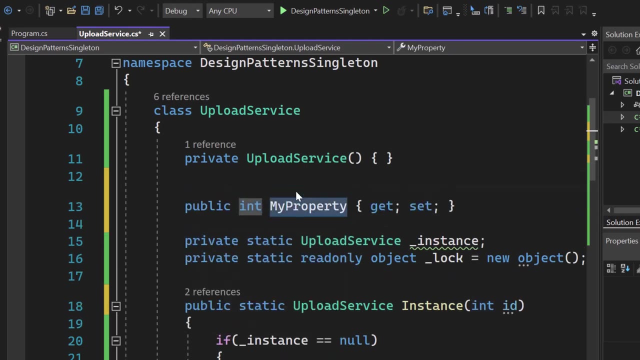 can really make a difference between between. well, the instances, right. so this is why we go into our instance here. let's simply add an integer here, let's call it ID, and right here at the upload service, let's set a property. let's call it prop, let's call it int ID. there we go. we can simply call get, we make private. 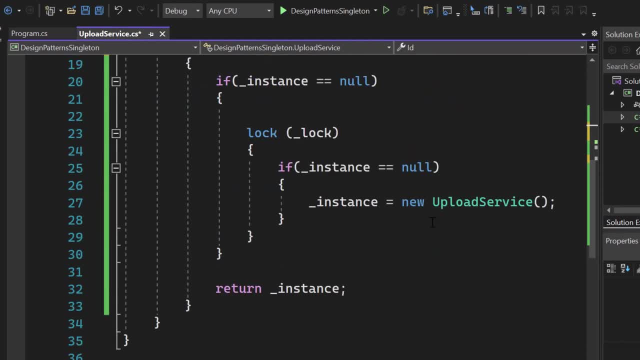 set. really, this is just for validation, so you can see that it's a little bit more complicated, but it's a little bit more complicated, but it's a little bit more complicated. so get private set and when? so get private set, and when we create a new instance, we want to take the 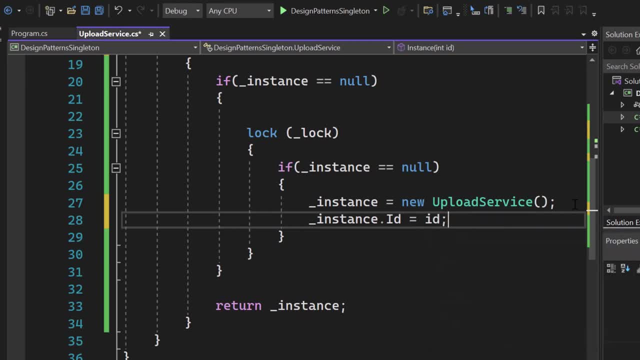 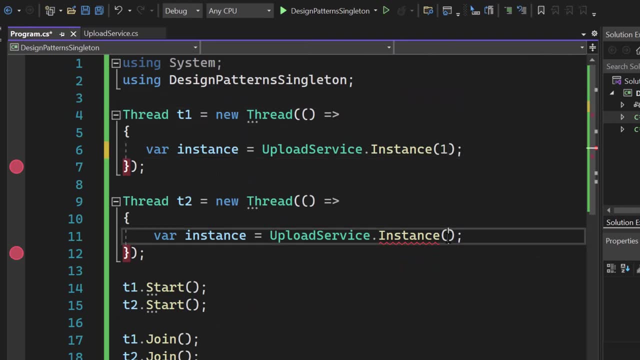 we create a new instance. we want to take the instance and set the ID to whatever instance and set the ID to whatever the user submits right here in the instance. the user submits right here in the instance method. so let's switch over to method. so let's switch over to the program. let's say this is instance ID 1. 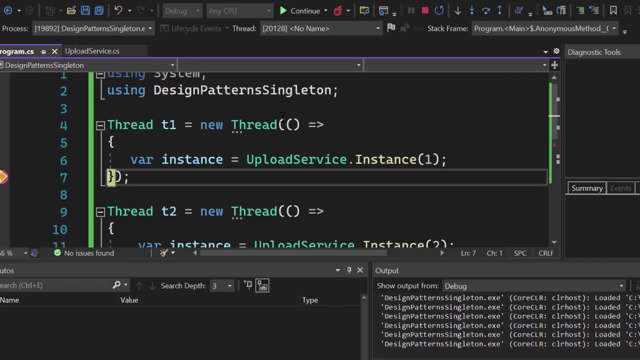 the program. let's say: this is instance ID 1 and this is instance ID 2 right now and this is instance ID 2 right now. let's hit start and basically both. let's hit start and basically both instances should be ID 1 right, because 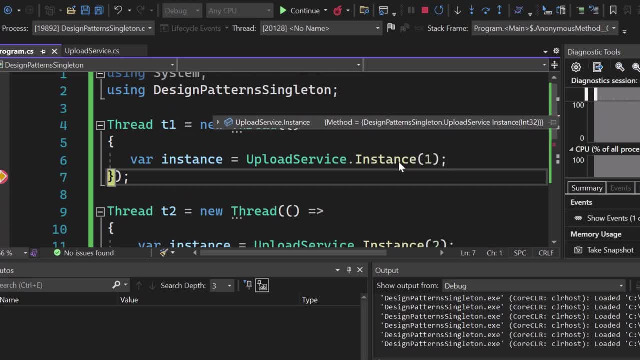 instances should be ID 1 right, because we create a upload service instance, we we create a upload service instance, we set in one and we call it a second time. set in one and we call it a second time instance and we sent in the two instance and we sent in the two. but that one should not create a new. 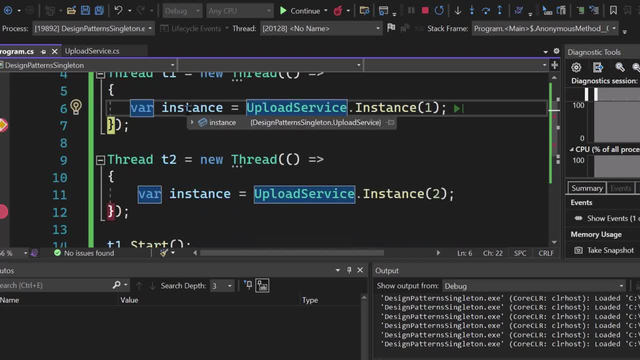 but that one should not create a new instance, so the first one should get used instance, so the first one should get used instead. so if we hover above instance instead, so if we hover above instance and we see ID 1, which is fine, perfect, and we see ID 1, which is fine, perfect, right, so let's press, continue. now we 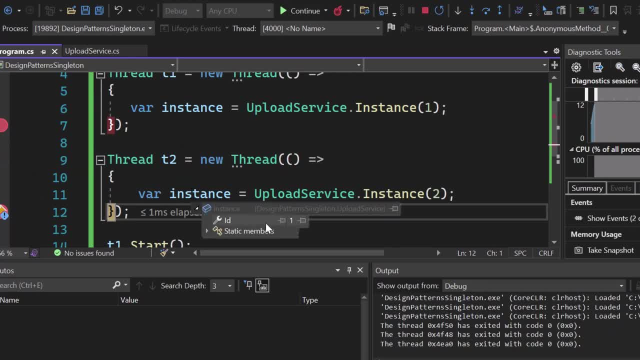 right, so let's press continue. now we come to the second breakpoint. let's take come to the second breakpoint. let's take a look at instance again and the ID is a. look at instance again and the ID is still one. if we take a look, we could see. 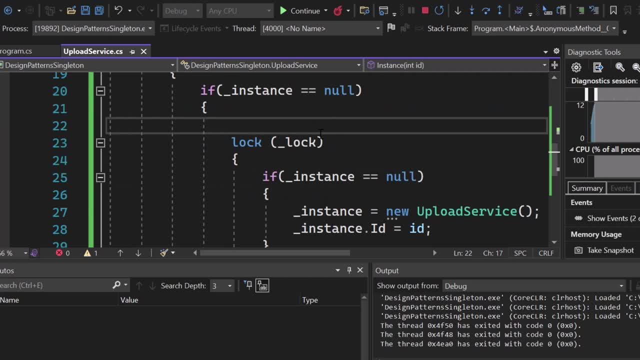 still one. if we take a look we could see: okay, the instance run into a lock. so we okay the instance run into a lock. so we waited at the lock with the second, waited at the lock with the second thread and the first thread created the thread and the first thread created the instance with ID 1. so our second thread. 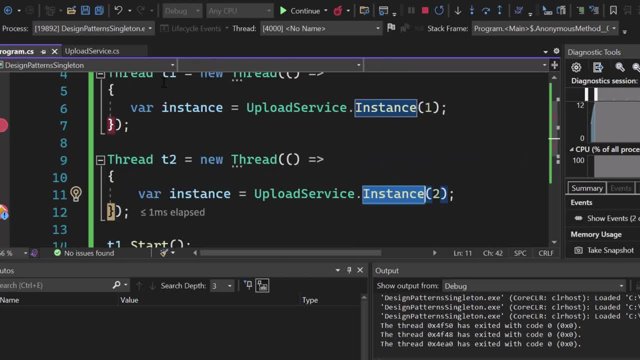 instance with ID 1. so our second thread created the instance with ID 1, so our instance with ID 1. so our second thread never created a new instance and never, never created a new instance and never set the ID. so this is the proof that set the ID. so this is the proof that, even though we have two separated threads, 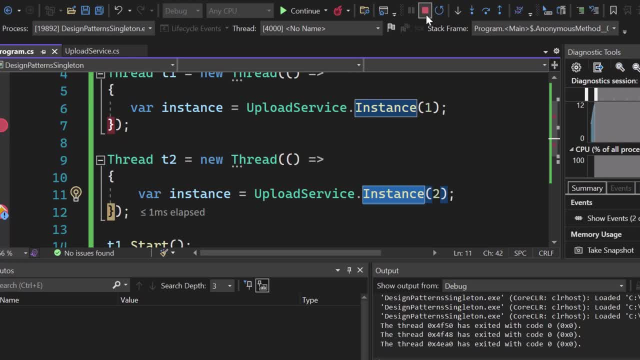 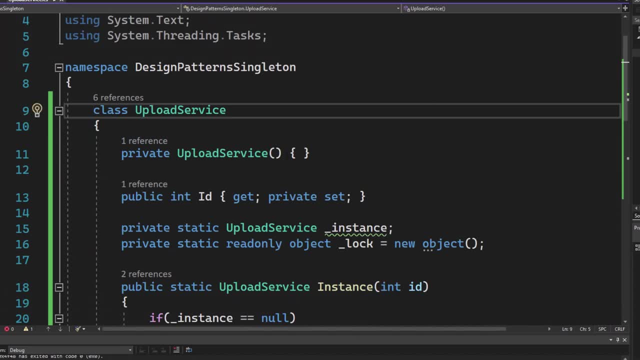 even though we have two separated threads, we have a single instance used in our. we have a single instance used in our application. now, now, at the very application, now now at the very beginning, I removed the internal access beginning, I removed the internal access modifier and I said we will replace it. 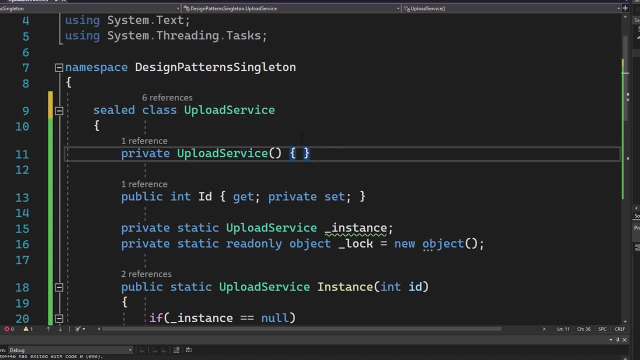 modifier and I said we will replace it and we will replace it with this sealed and we will replace it with this sealed keyword, which basically means that you keyword, which basically means that you are not able to inherit from that upload, are not able to inherit from that upload service, which makes again sure that we 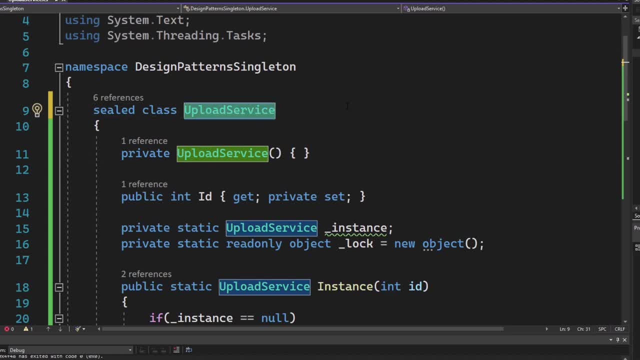 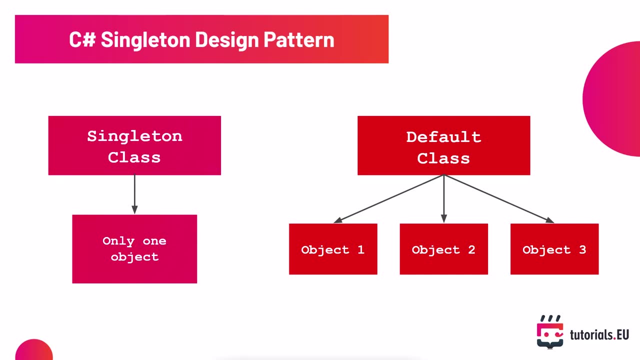 service which makes again sure that we only have a. only have a single instance of that class in our application- awesome. so now, single instance of that class in our application, awesome. so now you know how to apply the c-sharp. you know how to apply the c-sharp singleton software design pattern and, if you like,